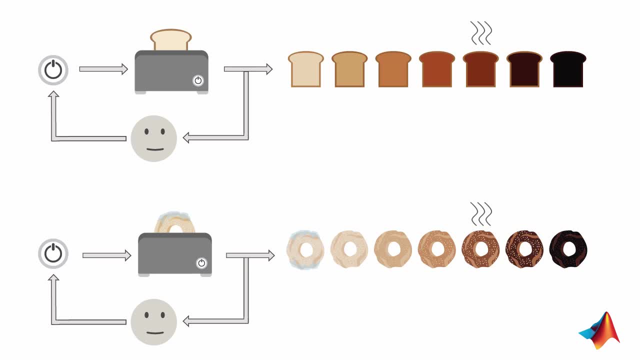 the toaster. This is the basic idea of Feedback Control. Let's try this on a slice of bread and a frozen bagel. You turn on the toaster and start monitoring your bread. When the toast reaches the color you want, you turn off the. 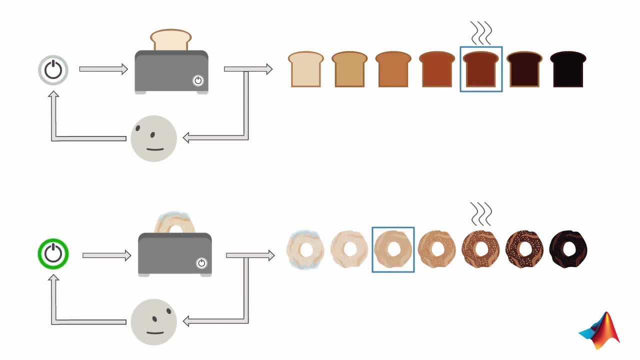 toaster. Notice that you didn't turn off the toaster. You can see that the bread is still on. You don't have prior information on how long to toast the bread. Monitoring them allowed you to tell when they have reached your desired color. so when to turn off the toaster. 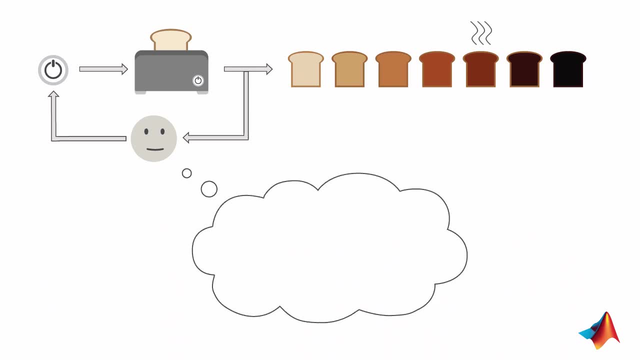 We will now read your mind. Don't worry, it's not to hack your accounts or anything, but just to reveal the complete Feedback Control structure. While you are monitoring the bread you draw, you plot in your mind: This is when you start monitoring your bread You have. seen that the bread is done. You're left with your hands shaking, Don't even try to read. Wait, It's still interesting how you got the right ouence of progress. You said not for the Empy ilea mate. It took the regarding story, as you're all eyes had at an obtained Addable. 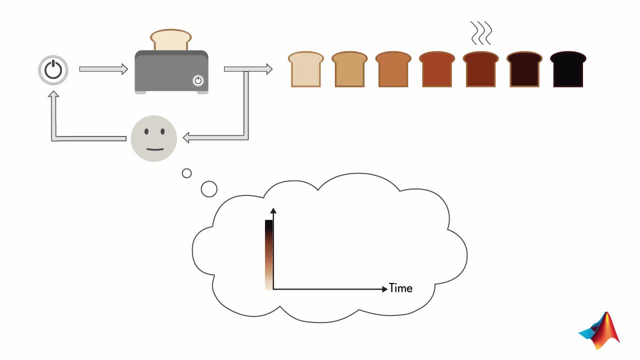 Let me point out someode. you're small, but close to your past lifetime, thanks to your mind. on the y-axis you have the bread color that you're watching and on the x-axis you have the time. this is what you want. then you start toasting and this is what you see at each time instant. you. 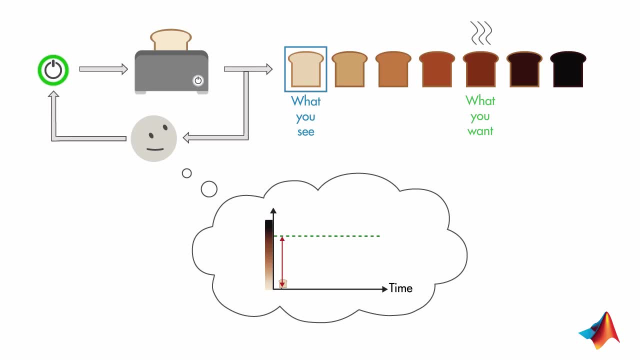 compute an error between what you see and what you want. if this error is not zero, you keep toasting. when what you see overlaps with what you want, the error becomes zero. your yummy toast is ready, so you turn off the toaster. if we now project what you think in your mind on to the closed 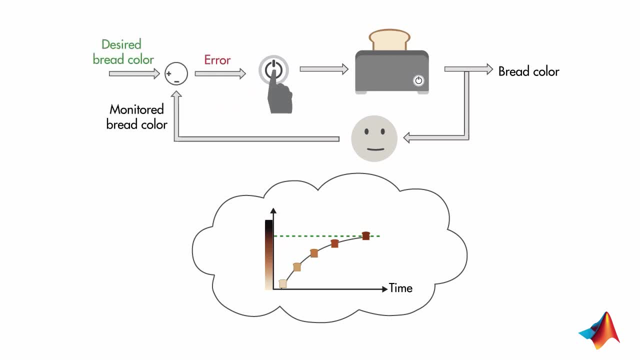 loop structure. here we get the complete feedback loop. this part represents the comparison you make between what you see and what you want. you compute the difference between monitored and desired bread color and this gives you the error. then, based on the error, you decide whether to keep the toaster on or turn it off. next we